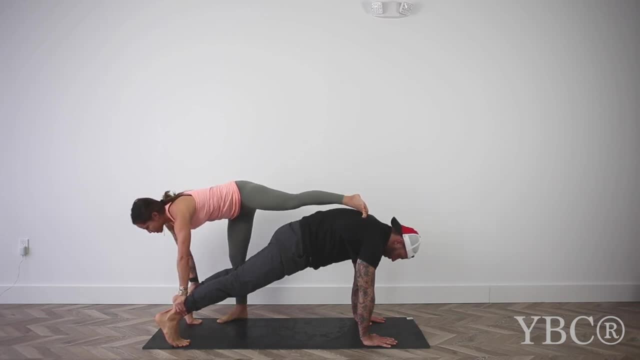 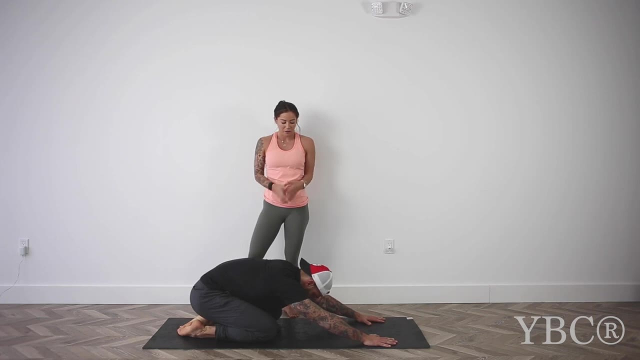 breaths And then you can step down if you're the top person, And the bottom person will come down into a child's pose. So for a child's pose you want to have your arms out in front of you. You can press into your forearms. You'll feel a really nice stretch through. 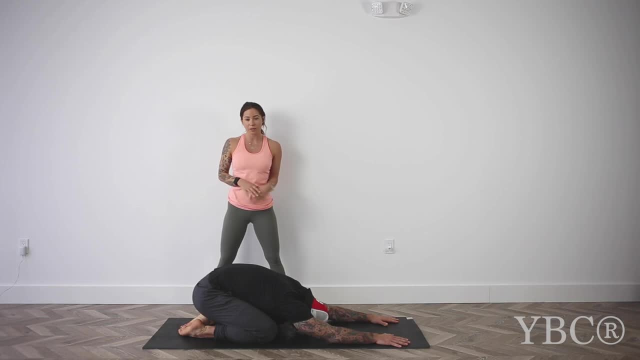 your armpits, Reach your hips back towards your heels and the head will be down into the ground. If you have a small child who's been running around all day, then they're probably super, super mobile- much more mobile than we are, So they can probably come onto. 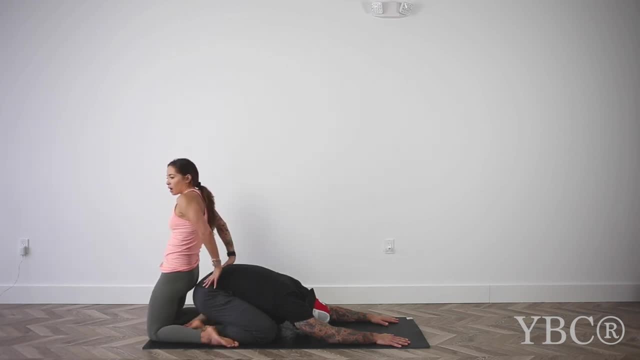 their shins, send their hips on your hips and then lift up And then lean back and lay over you. Don't go into that cold. If you're an adult trying to do that, don't go into that cold because it won't feel good. Then the arms can hang. 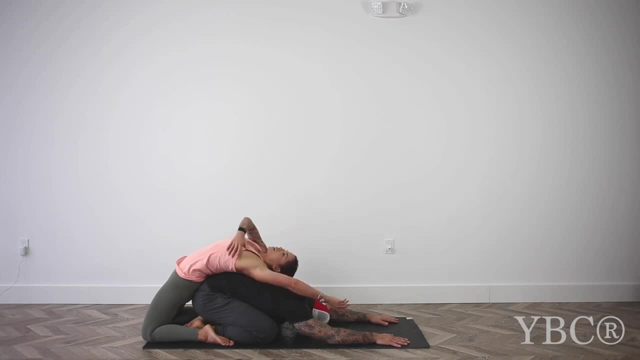 out to the side or reach up to the sky and it just has a really nice heart opener here. The other option is- and this one is a little less intense- is to just keep the feet out in front of you as you squat down and then step back, And usually it feels pretty good. for the person on the bottom. But if you're a child, you want to be able to lean back and lay over you. Don't go into that cold. If you're an adult trying to do that, don't go into that cold. 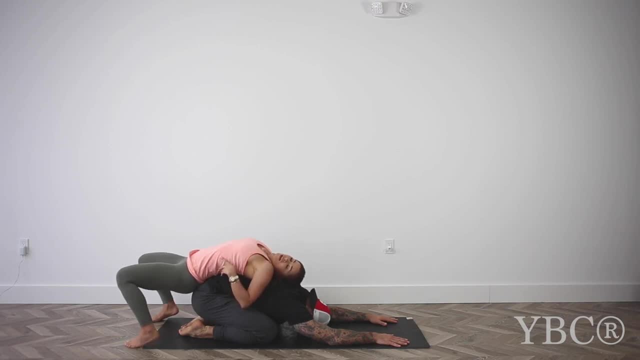 Yeah, it's just like a really nice assist for them, And so you can breathe a couple breaths here And then, when you're ready, you can release. So the top person will come off and the base will come into a downward facing dog. For a downward dog you want to. 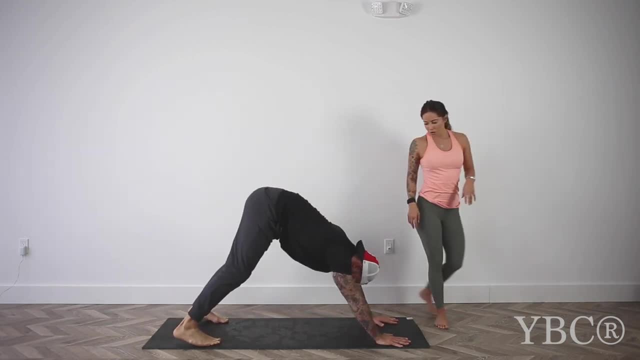 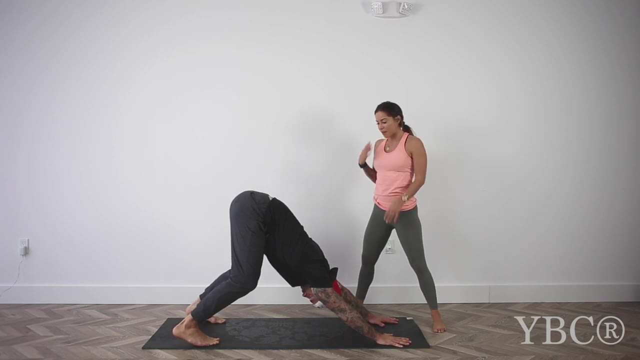 have your hands shoulder distance. You want to push the ground away so that you have really long armpits. Make sure you're plugging into all four corners of the palms. Let the head hang heavy. Your knees can bend. You want to reach your hips up and back. Belly goes. 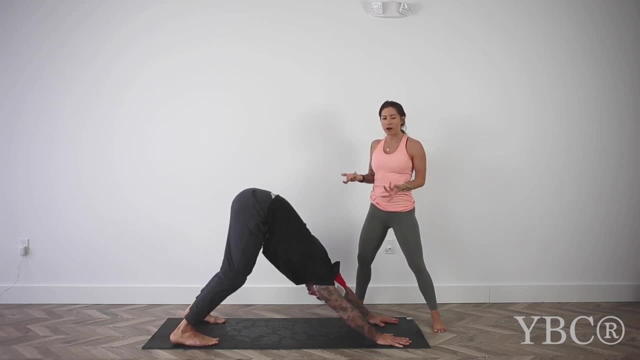 towards the thighs And then press the heels down towards the ground. But if they don't get there, no big deal. Now, if your knees are bent a whole lot and your heels are way off the ground and you're really super tight through your hips, like if this is kind of 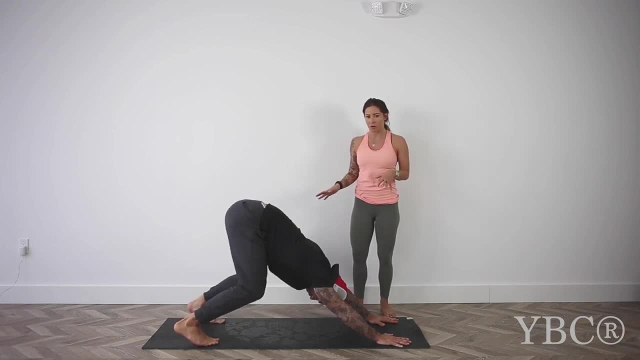 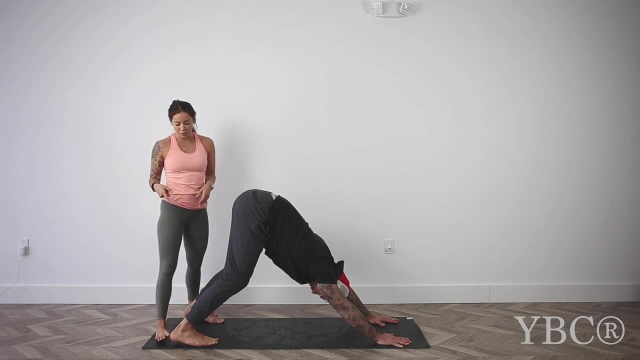 what your downward dog looks like, then this probably isn't the best pose for you, But if you know that you're very, very close to the ground, then you're going to be able to do this. If you're very, very close, like Dan is, with the heels towards the ground or 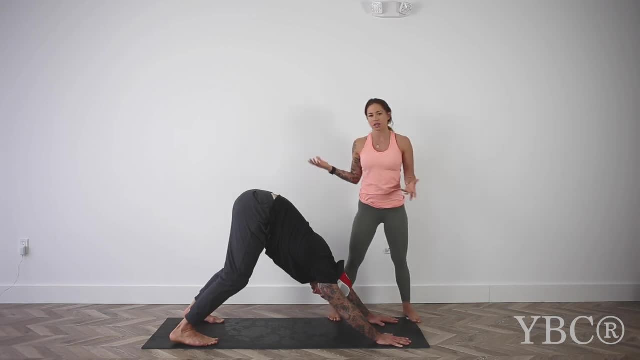 you're there, then you can safely do this. My only hesitation is like if the top person is kind of heavy and they push into you and your heels are like way off the ground, it might be too much on your hamstring, So use caution with this. Then, from here, the top. 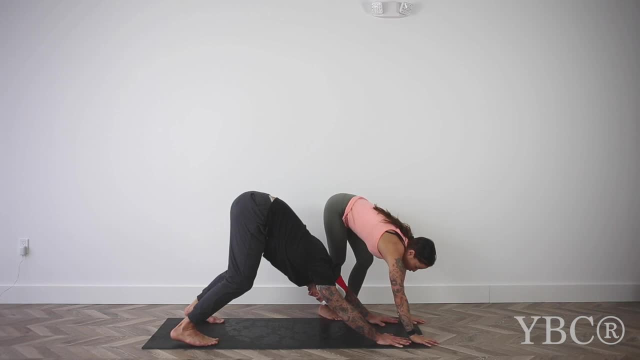 person is going to take their hands just in front of the base's hands and they'll take their toes to the low back. Is that all right? Yeah, And they will kind of press in and lift up. You're going to push the ground away. 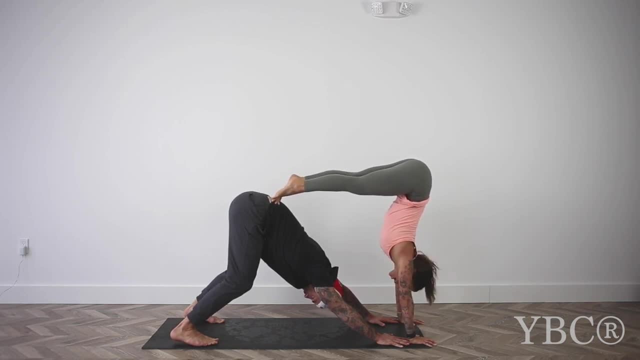 You want to feel that your hips are over your head- I can't really see, I think they are- And then you can also play around with the arm balance here if you want. So you can take one foot up, lean into it a little bit, Think about cartwheeling out of it if you don't. 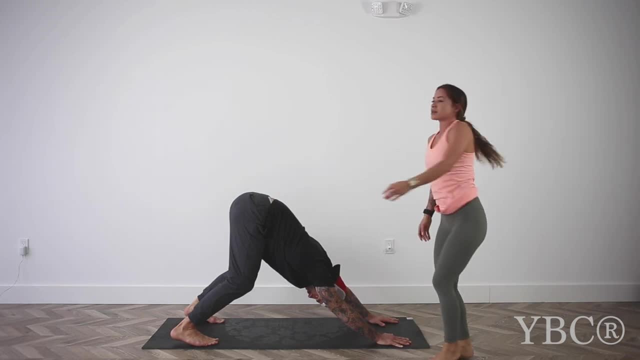 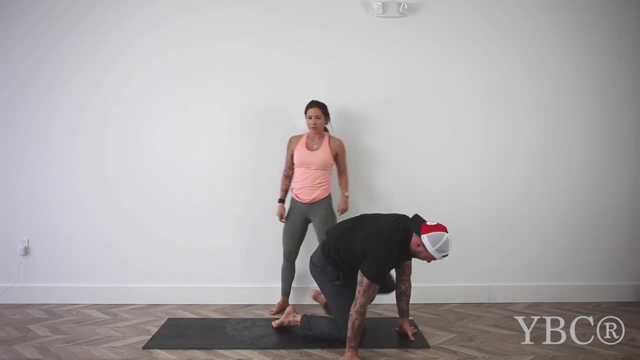 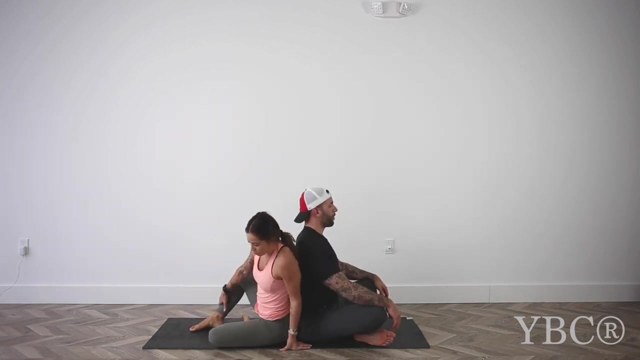 have your balance And if you want to get out there, you go From here. your person, your base can come down into a seated position, sitting in like a crisscross leg position, And the other person will sit up against their back And just take. 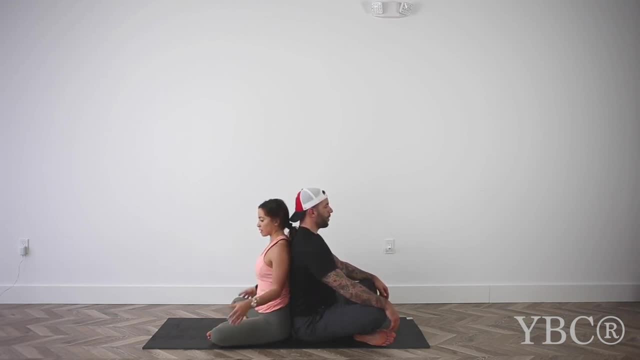 a breath. here You can kind of feel your upper back against their upper back And you can breathe in together, feeling the expansion through your ribs. You can do that one more time: Big breath in And then take your right hand and your partner will take their right hand, You'll take your. 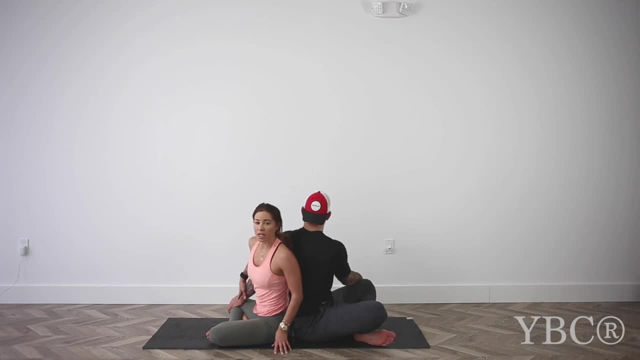 right hand to your left leg. Your partner will take their- sorry, their- left hand to your opposite knee And you will twist So big breath in, Grow, tall, Exhale. You can use your partner's leg a bit to leverage a deeper twist.